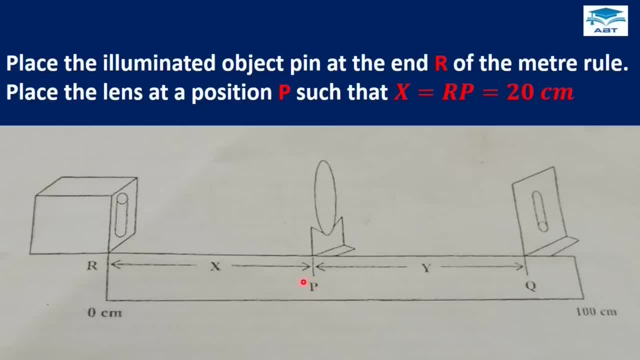 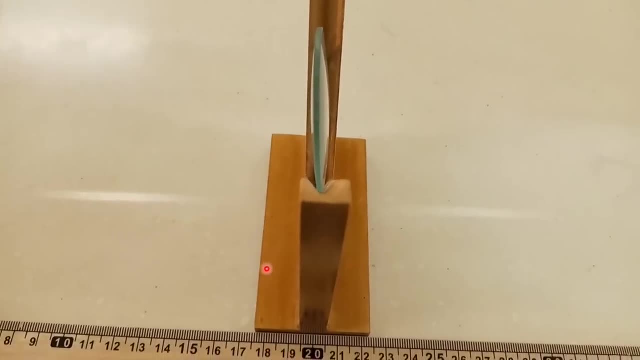 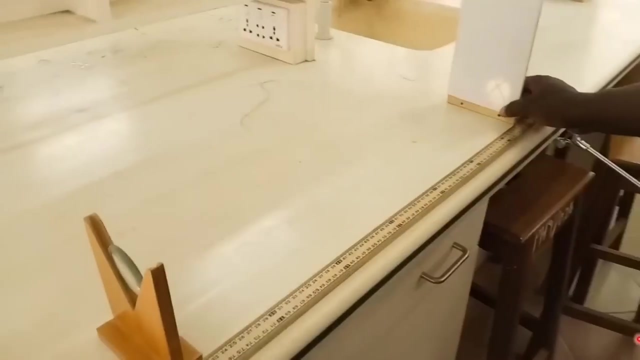 position P, such that the distance between the ray box and the center mark of the lens holder is 20 centimeters and the screen will be at this side. So we place the center of the lens at 20 centimeters from the ray box and move. 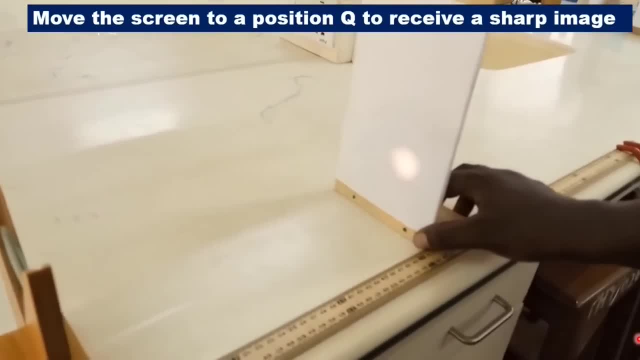 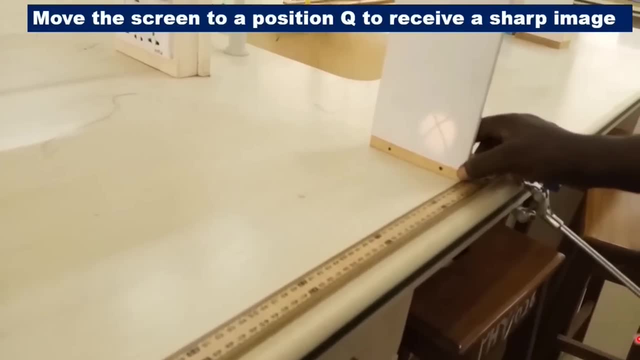 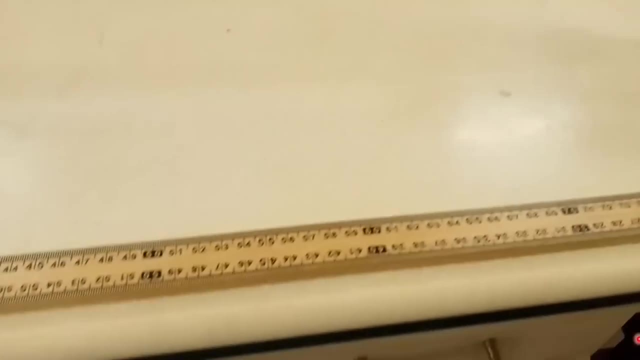 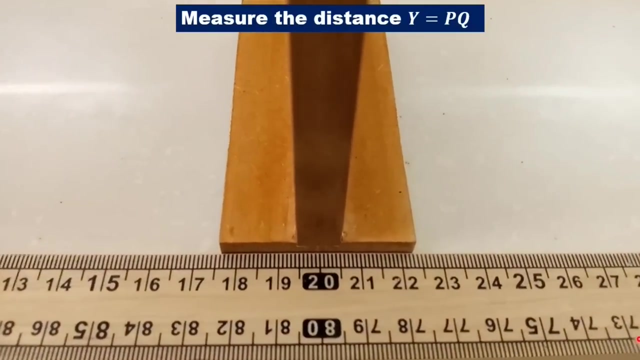 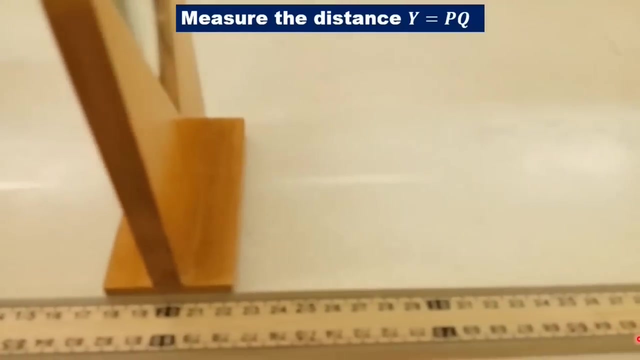 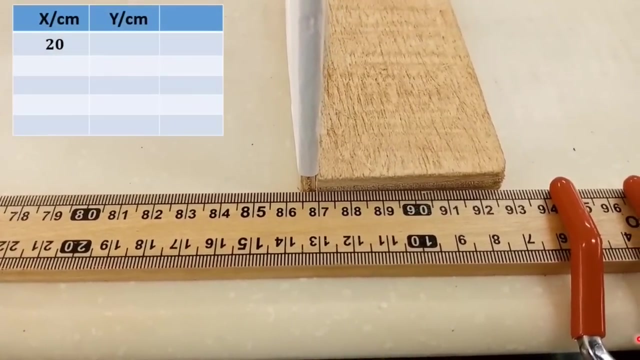 the screen to receive a sharp image, And we measure the distance between the center of the lens and the screen. The center of the lens is at 20 centimeters and the screen is at 86.4 centimeters, So we solve the problem. 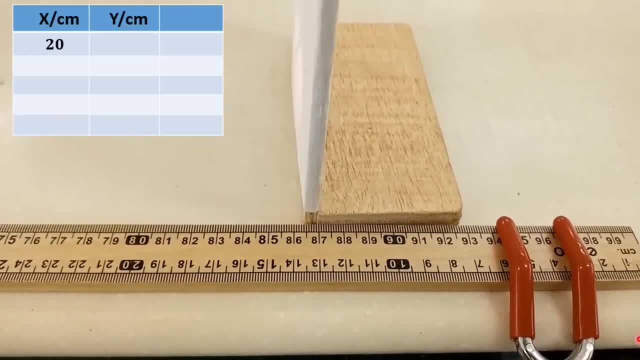 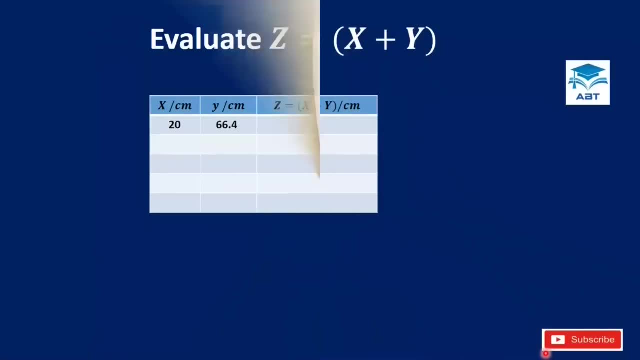 subtract 20 centimeters from 86.4 centimeters and then Y is 66.4 centimeters. At this part of the question we are to evaluate Z equals X plus Y. So 20 centimeters plus 66.4 centimeters equal to 86.4 centimeters. 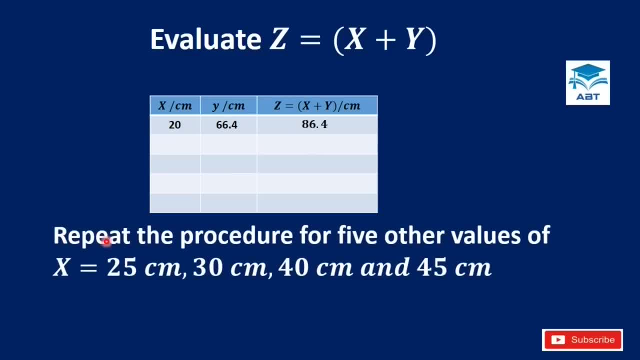 And we are to repeat the procedure for five other values. of X is equal to 25 centimeters, 30 centimeters, 40 centimeters and 45 centimeters, And in each case we workout the volunteers on the X and Zzonyn's microscope to predict. 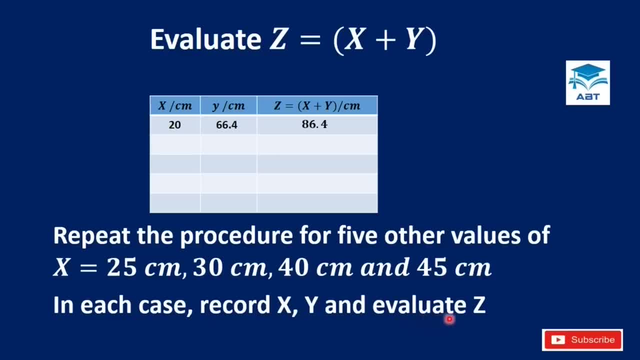 value of x, y and evaluate z. So we are going to set the center of the lens at 25 centimeters, locate a sharp image and record the value of y, add x to y and then do the same thing for 30 centimeters, 40 centimeters and 45 centimeters. 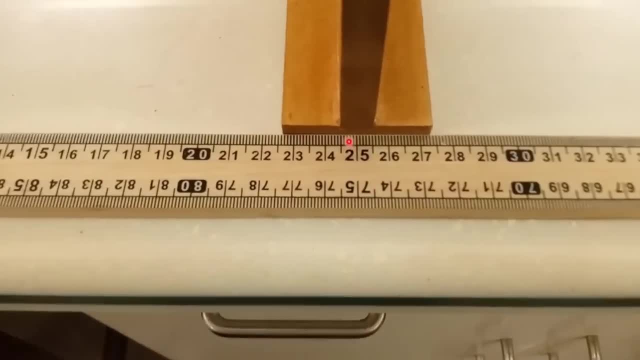 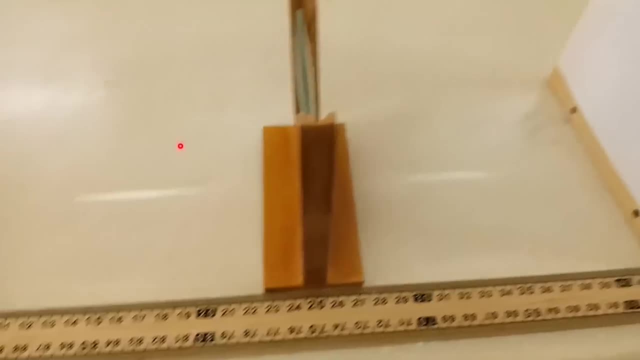 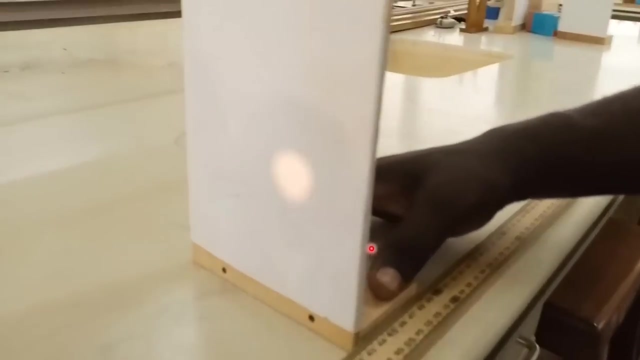 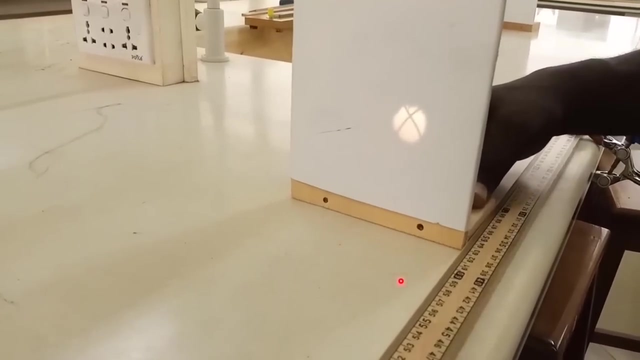 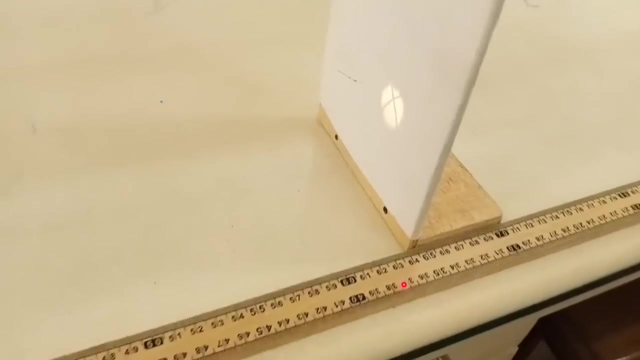 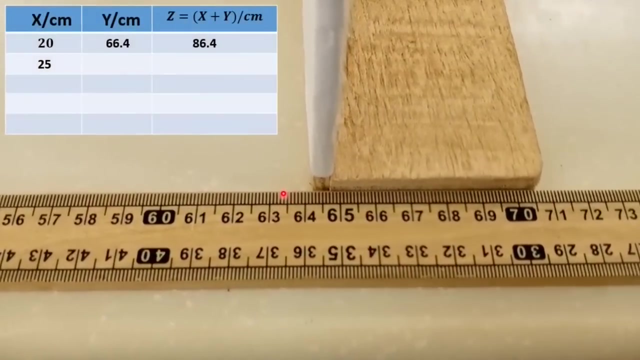 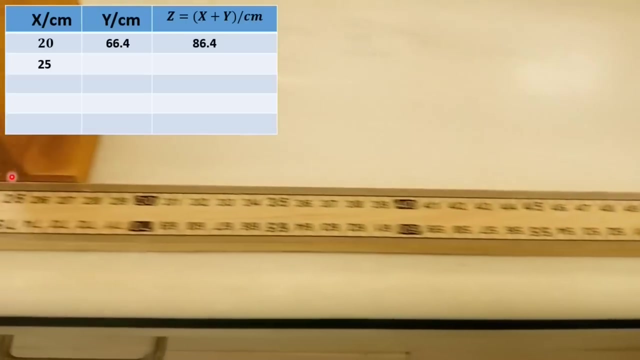 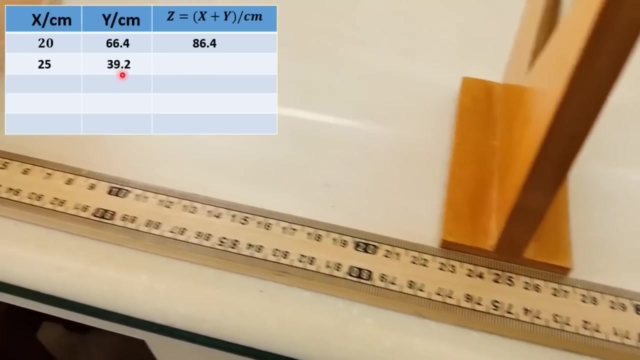 So we place the center mark of the lens holder at 25 centimeters from the ray box and adjust the screen to receive a sharp image. So we have a sharp image at 64.2 centimeters. So we subtract 25 centimeters from 64.2, and we have 39.2 centimeters. 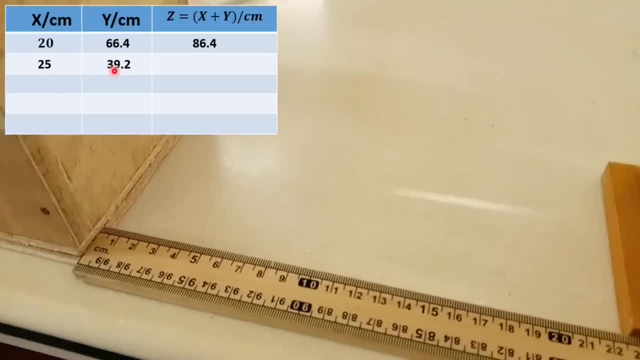 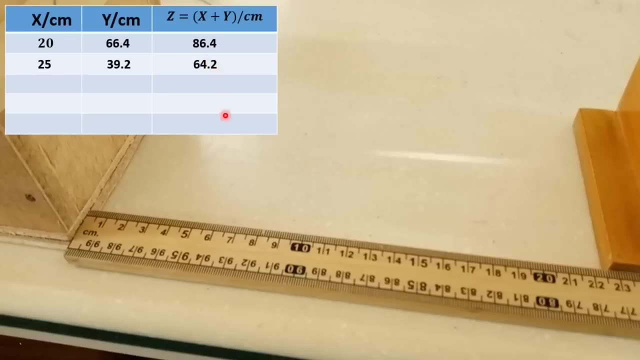 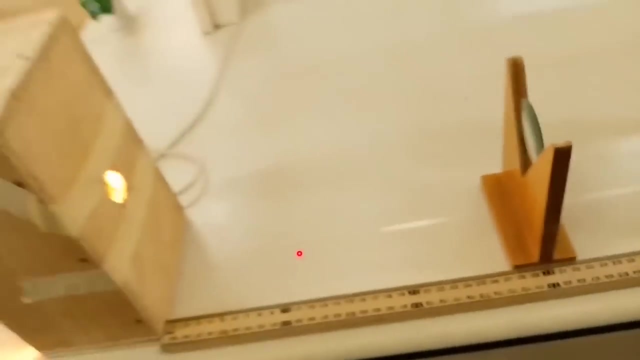 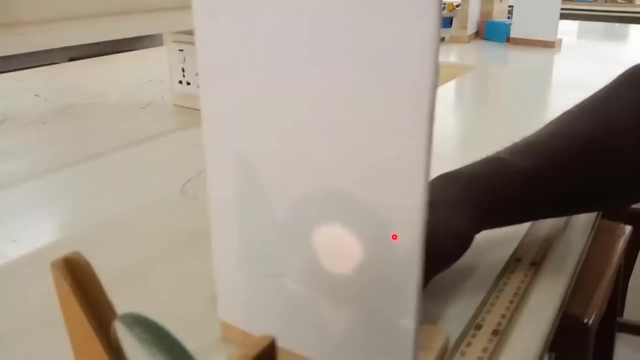 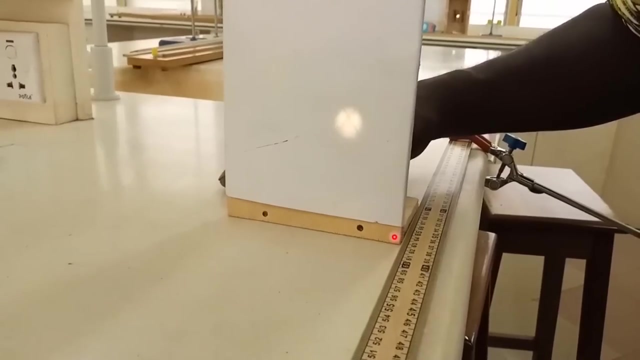 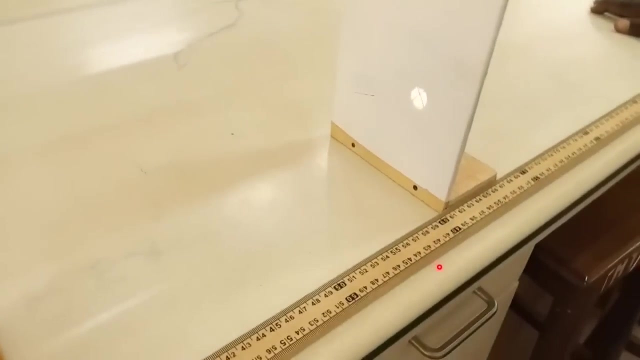 And 25 plus 39.2.. We'll give us 64.2 centimeters. Again, we place the center mark of the lens holder 30 centimeters from the ray box, move the screen to receive a sharp image. So we have a sharp image at 61 centimeters. 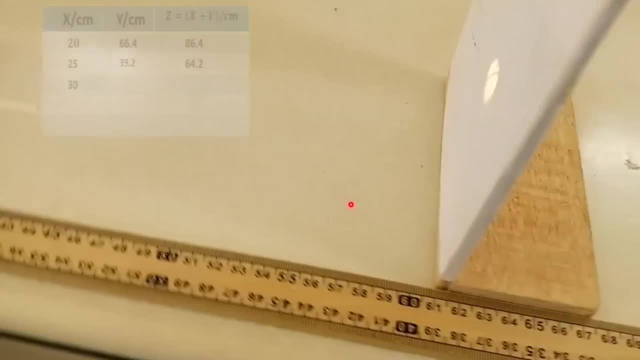 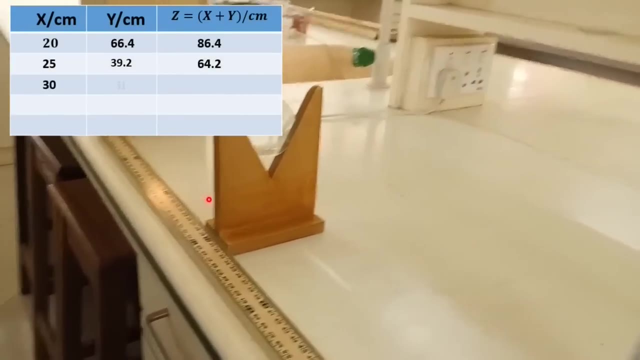 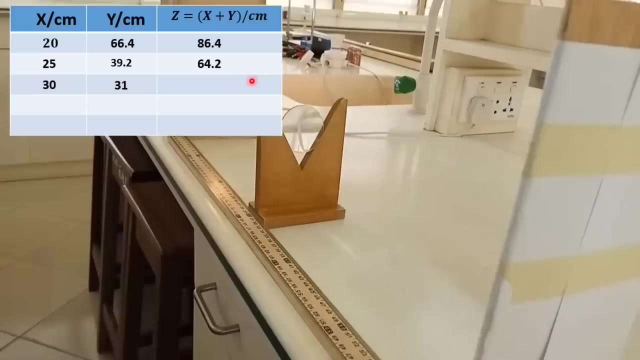 So we subtract 30 from 61, and we have 31 centimeters. And 30 plus 31 will give us 61 centimeters. So we place the center mark of the lens holder and adjust the screen to receive a sharp image. 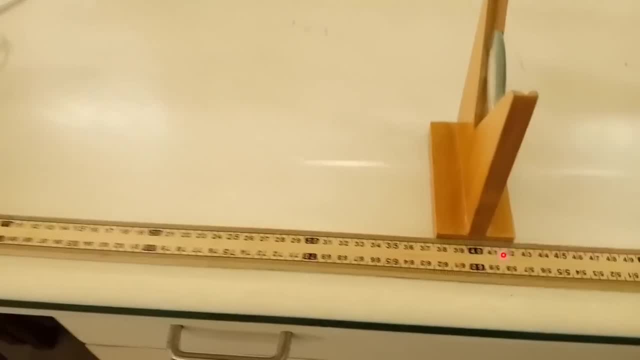 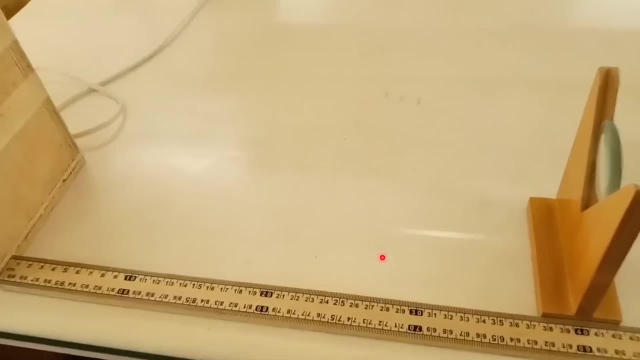 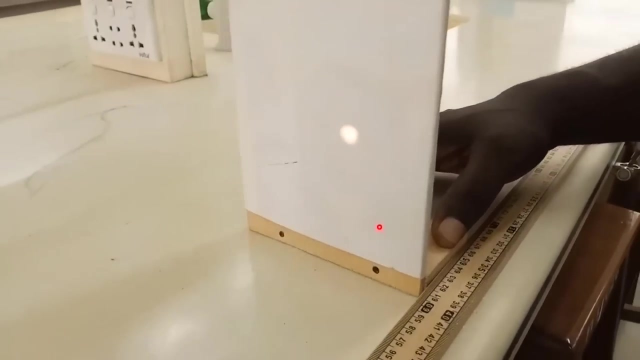 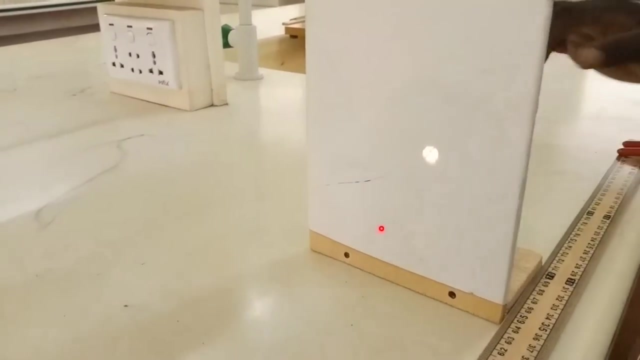 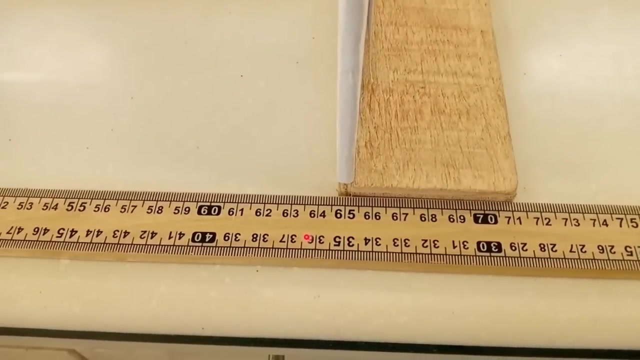 And one more. Yes, I am waiting. I have off camera Now black. I am waiting for���s center of the lens at 40 centimeters from the ray box. Adjust the screen to receive a sharp image. So we have a sharp image at 64.7 centimeters. We. 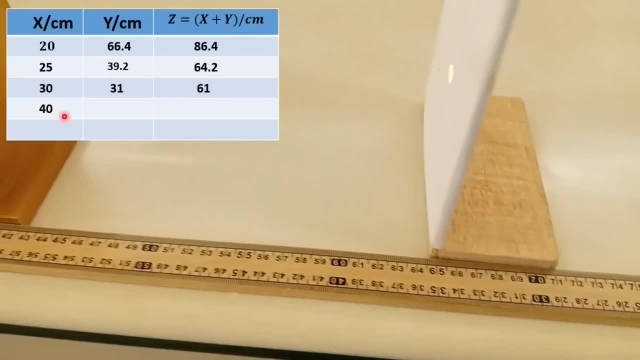 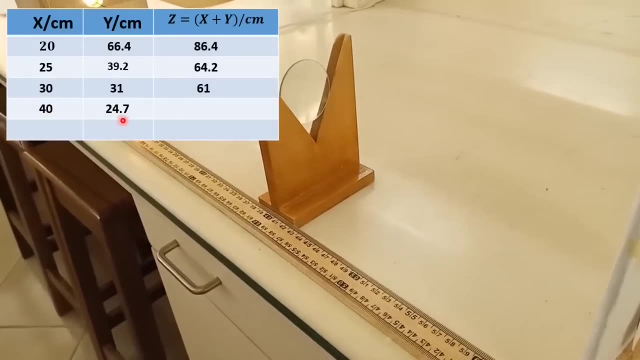 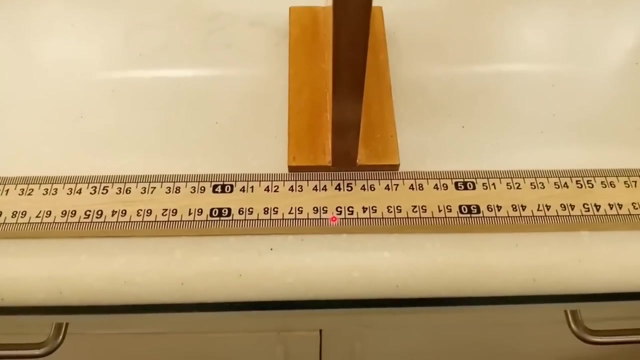 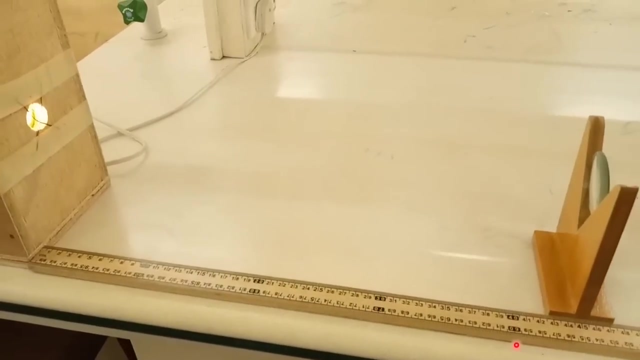 subtract 40 from 64.7 and we have 24.7 centimeters. We add 40 to 24.7 and we have 64.7 centimeters. Finally, we place the center of the lens at 45 centimeters from the ray box and adjust the screen to receive a sharp. 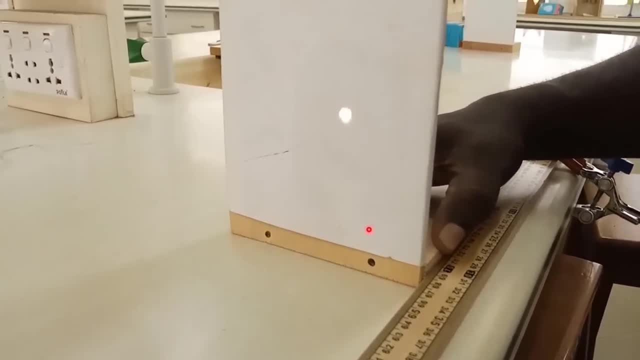 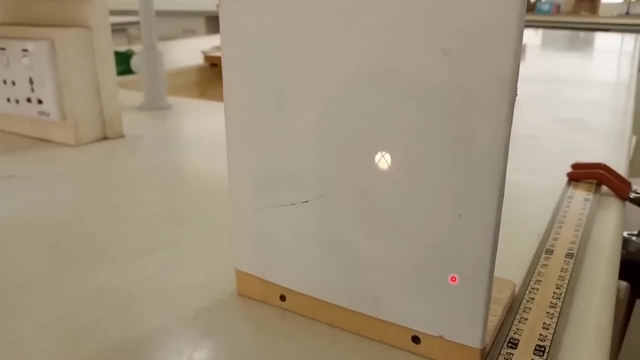 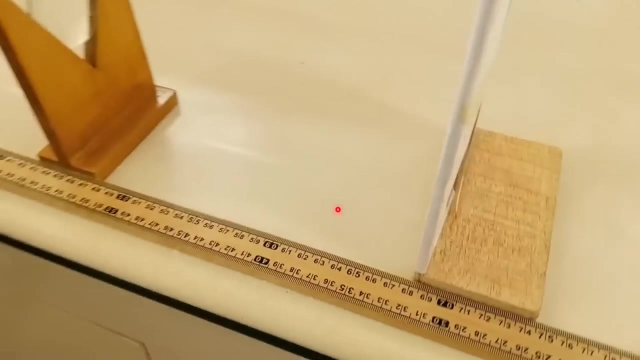 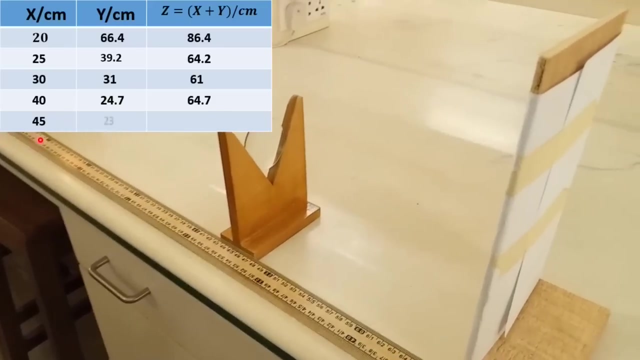 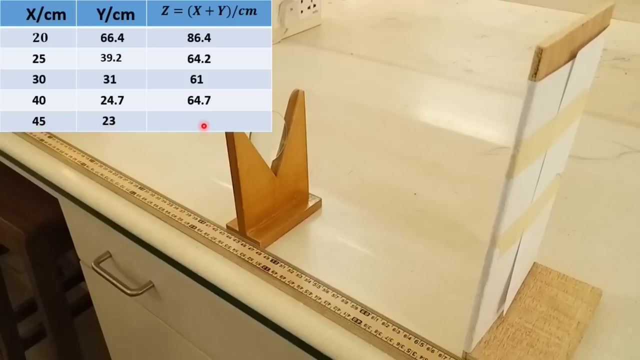 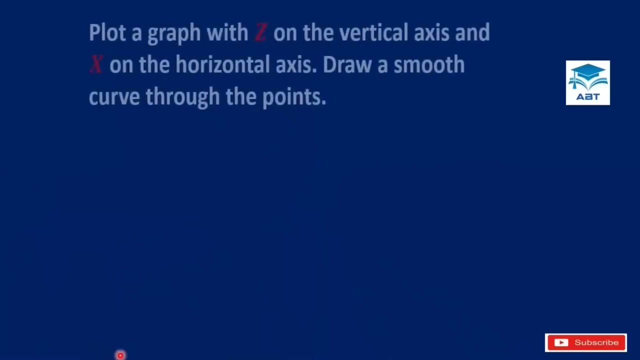 image. We have a sharp image at 68 centimeters. So we subtract 45 from 68 and we have 23 centimeters, and we add 45 to 23 and we have 68 centimeters. we are going to plot a graph with Z on the vertical axis and X on the. 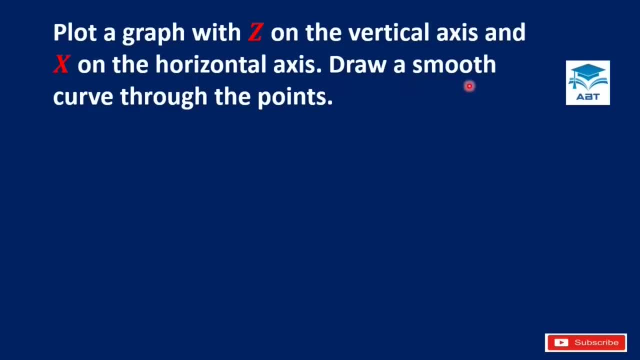 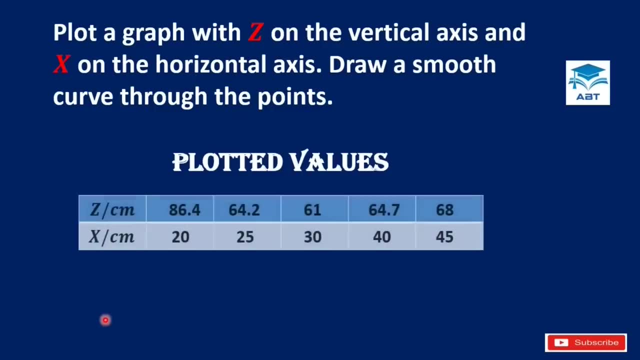 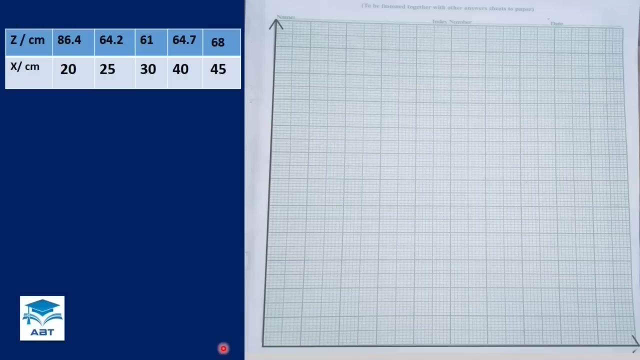 horizontal axis and then draw a smooth curve through the points. so we have our plotted values, the Z values and X values, all in centimeters. So So we draw our axis. We are going to plot Z on the vertical axis and X on the horizontal axis. 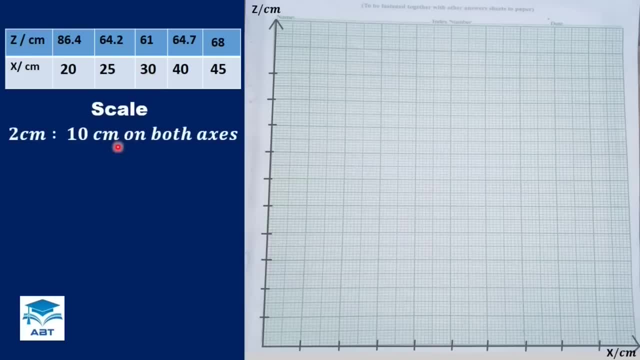 We choose a scale looking at the values. a scale of 2cm, representing 10cm on both axis, will be ok. So we start with 10cm, 20,, 30,, 40,, 50 and so on on the Z axis. 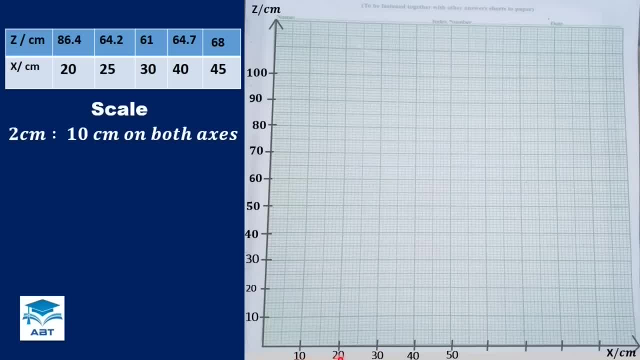 And then on the X axis too, we have 10,, 20,, 30,, 40,, 50,, 60, and so on. Each 2cm box has 10 divisions, so one small box represents 1.. Our first point: we have 20cm on the X axis, that's it, and 86.4cm on the Z axis. 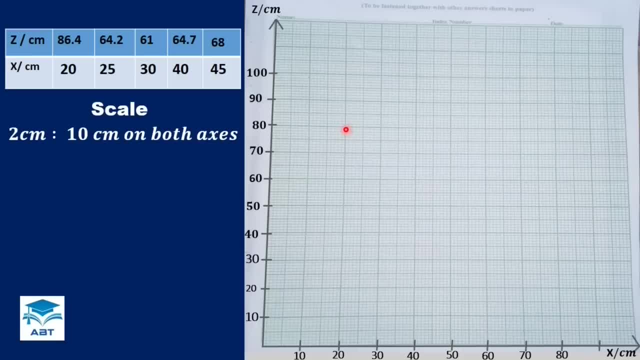 So we have 80 here. We count 6 boxes And then 0.4 go into the next box a little bit. The next point is 25cm on the X axis, which is here the middle of 20 and 30.. 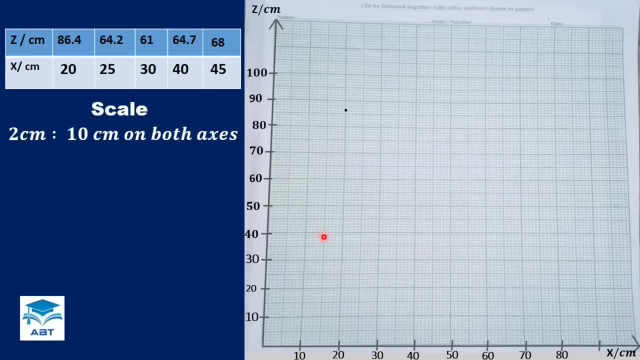 And 64.2cm on the Z axis. We move to 60, count 4 boxes And then move a little bit into the next box. We move to 60, count 4 boxes And then move a little bit into the next box. 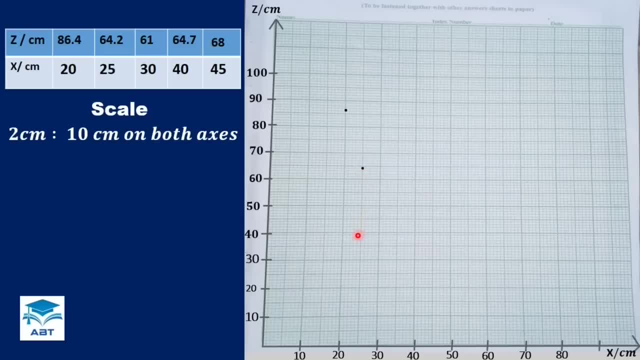 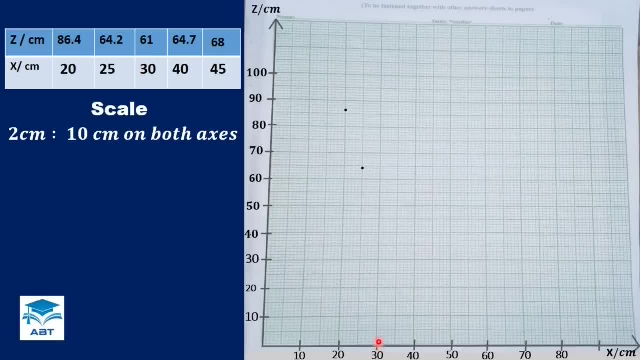 We have 30 on the X axis and 61cm here. The next one is 40, 64.7cm. We have 40 here 60. we count 4 and move into the next box. The next one is 60, 64.7cm. 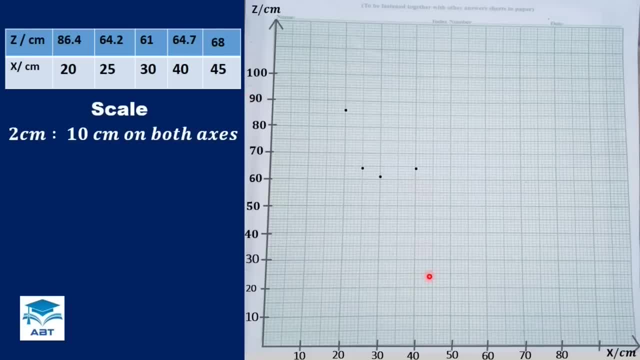 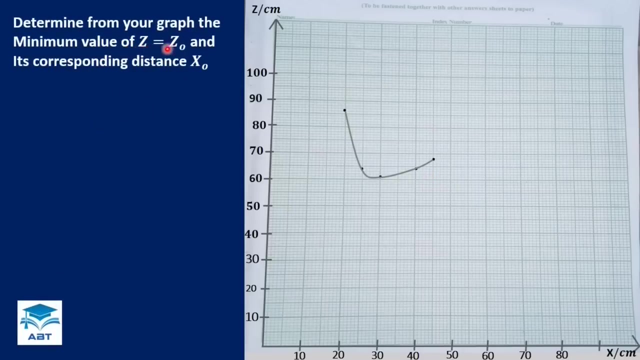 We have 40 here, This is 60.. one is 45.. 45 is here and 68. and we have the point here and we draw a curve passing through all the points. Determine from your graph a minimum value of Z equals Z naught and its corresponding distance, X naught. So this is the minimum.